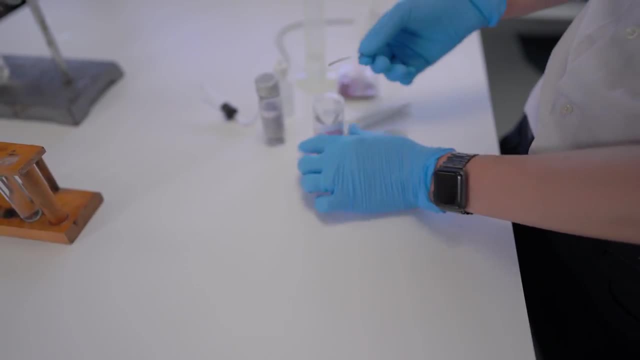 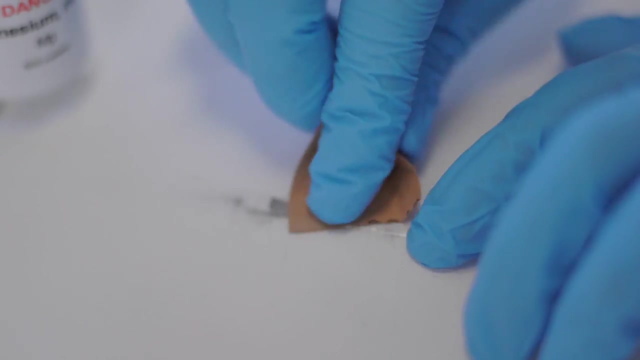 back to the bench. Here I've got some magnesium and these are magnesium ribbons, and you can see that it has a bit of a dull shine because it tends to react with the oxygen in the atmosphere. We're going to clean it off in a minute with some sandpaper, just to. 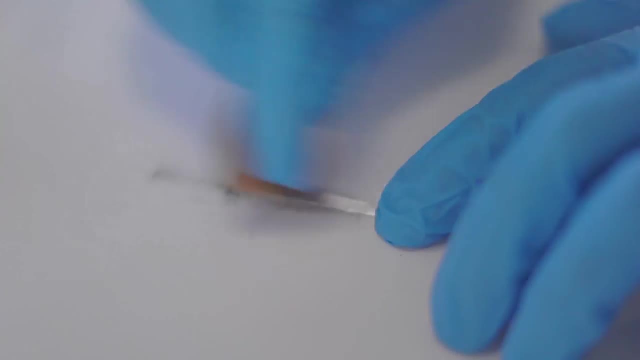 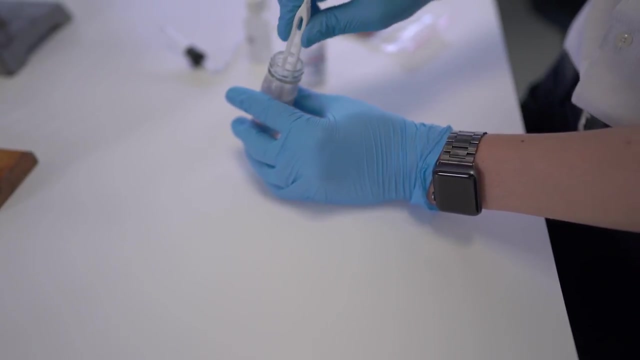 expose the bare metal and that'll allow it to react a bit better with the water when that happens. We also got some calcium here. Calcium here is quite a bit more vigorous in terms of reactivity. so we've got a jar here and we've got very tiny pieces, So these ones are probably not going to. 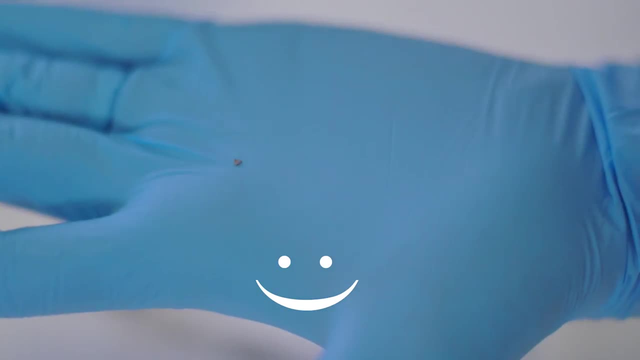 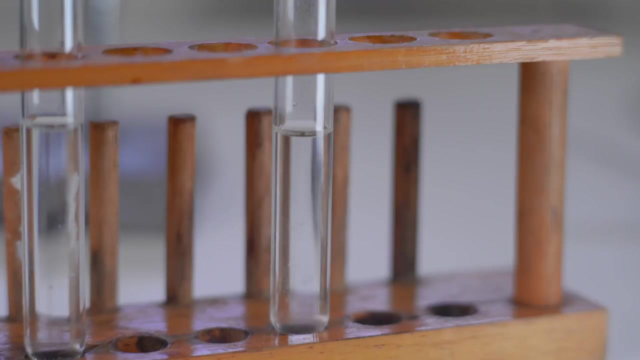 show up on camera. so we're going to switch our camera to macro mode in a minute so we'll get a close-up. So let's do our first test here with magnesium. We're just going to drop it into some distilled water, so there should be no impurities in here. So we're just going to drop this in and 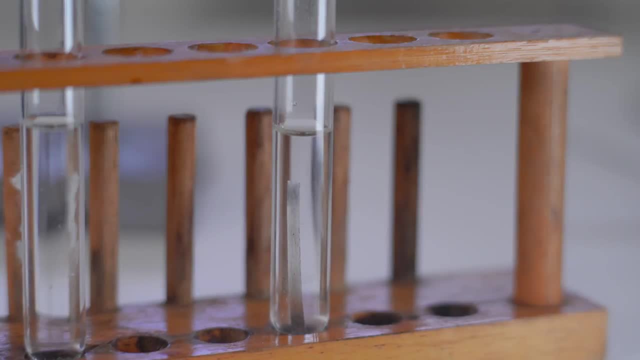 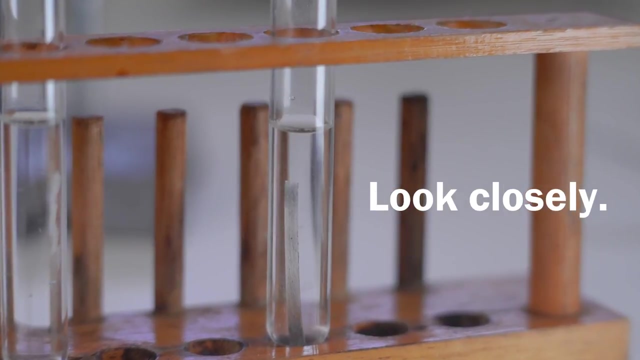 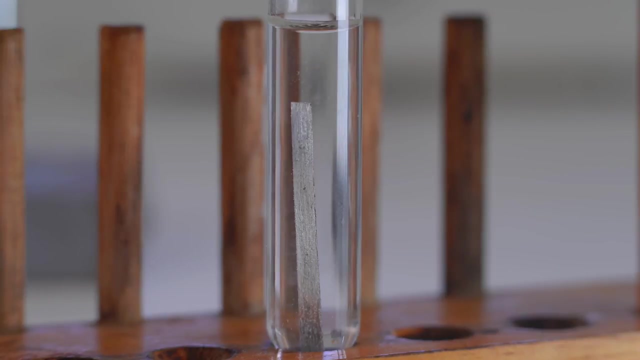 we're going to observe what happens for the next five minutes. Now that we have a close-up view, I think you'll find that there's quite a lot of these micro bubbles all over the surface, and so we definitely have a reaction going on here. So let's sort of 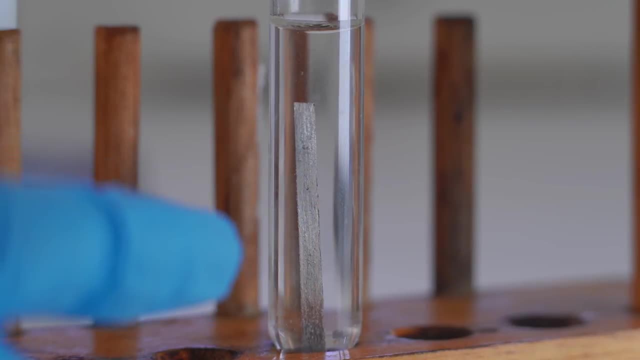 unpack what the reaction is. Well, the reaction is that the water is going to be a little bit more viscous. The magnesium is reacting with the water, which is H2O, so two parts hydrogen and one part oxygen, and the magnesium is sort of displacing some of the hydrogen atoms out of the H2O molecule. 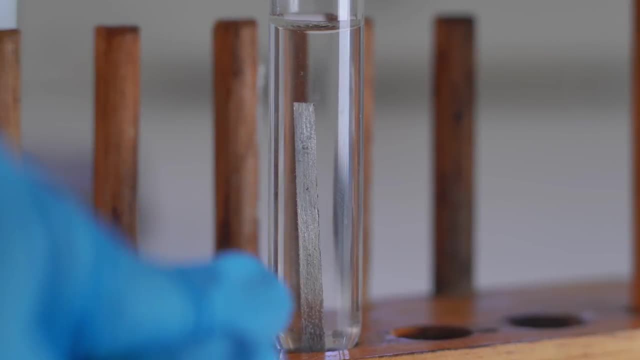 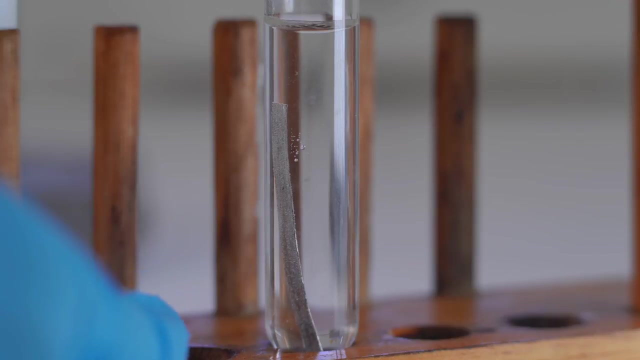 and so these, you know, ejected hydrogen atoms. they are forming hydrogen gas molecules, which is the gas bubbles we see on the surface: H2- that's what hydrogen gas is made from, and the remaining parts of hydrogen that hasn't been ejected. that's going to leave behind some hydroxide ions, which is known. 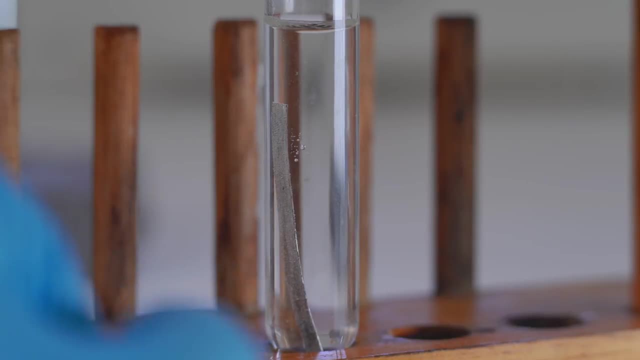 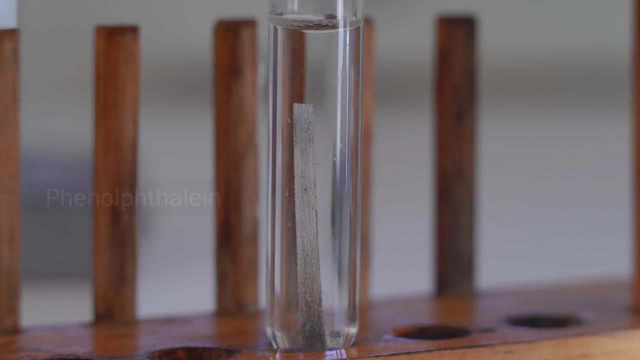 as OH-, and if you have a lot of these or very few of these present in the solution, that's going to affect the pH, the level of acidity of the solution. Okay, so it's been about five minutes and now we're going to give it a pH test. So what we're going to add in here is a chemical we call. 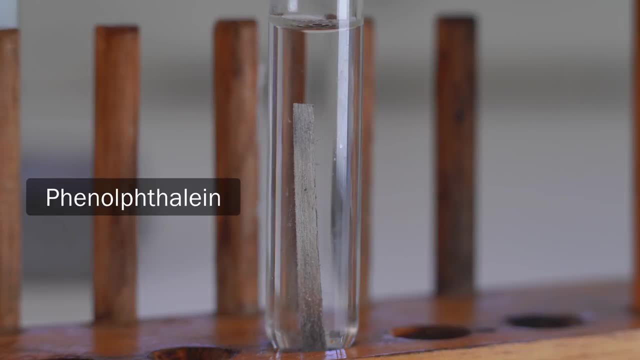 phenolphthalein, and this is a pH indicator. It tends to change colour vibrantly at a certain pH range. So if the pH, which is a measure of acidity, if the pH is neutral, so pH of 7, right in the middle of the scale. in fact, the scale goes from 0 all the way up to 14.. 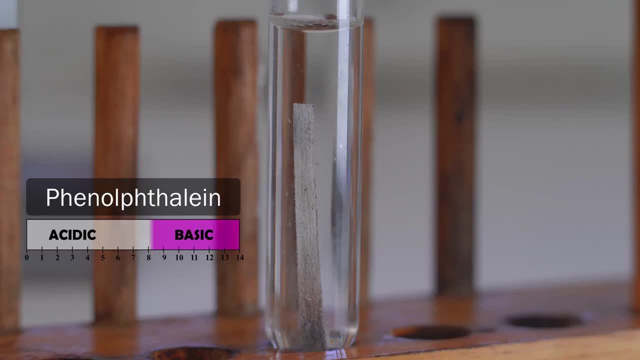 So 7 being exactly in the middle. it's a neutral, so ordinary tap water should be around pH 7.. If you're anywhere between 0 and about 8.3 on the pH scale, this chemical will just be colourless. However, if it's higher than 8.3, 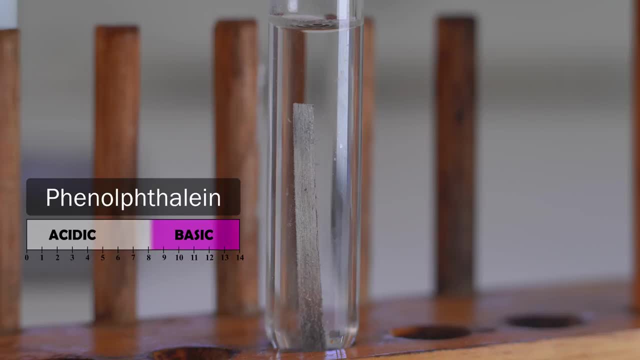 so it's well and truly into the alkaline solution territory. we should see a very strong pigment of pink, So let's give it a few drops. Okay. so we haven't seen any chemical change there, so it should go pink because we should be making an alkaline solution. So what's probably happening here is that our reaction. 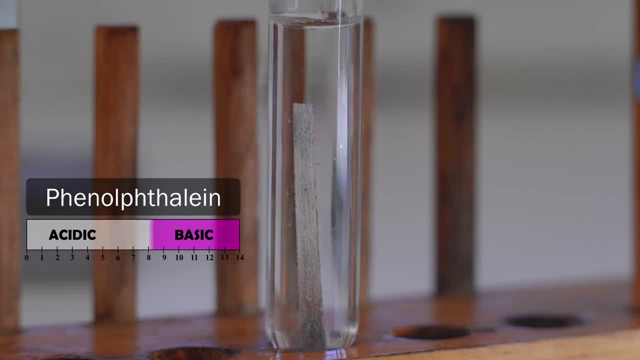 here is just going so slowly that we haven't had time to develop enough of the OH- ions to get the pH of the whole solution to increase to 8.3.. What we can do is we can grab this test tube and we're going to put over a Bunsen burner just to warm it up a bit. So the reason why adding: 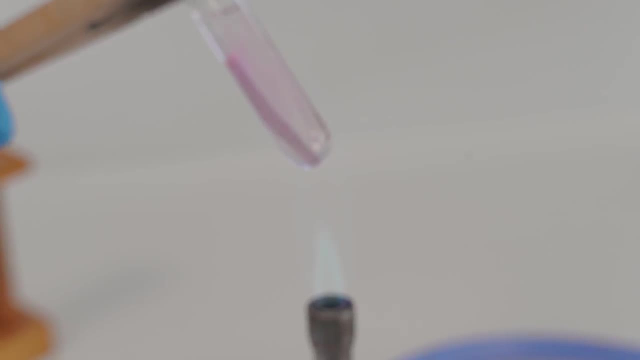 heat makes this thing happen a bit faster is because you add energy to each of those molecules of water to react with that magnesium. so we're getting a bit more contact between the two chemicals, the two substances, and we're starting to see this pink colour develop. so that's the indicator that I was speaking to you about earlier. Now we're going to turn our attention to the water. 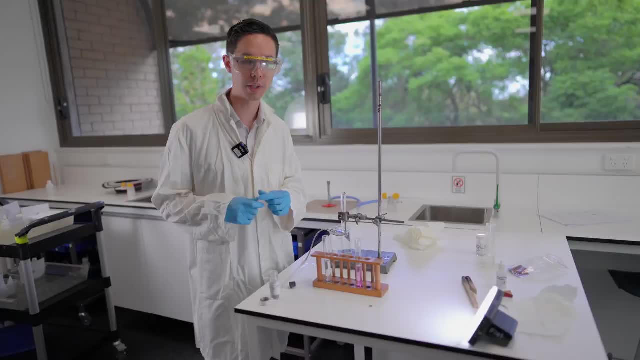 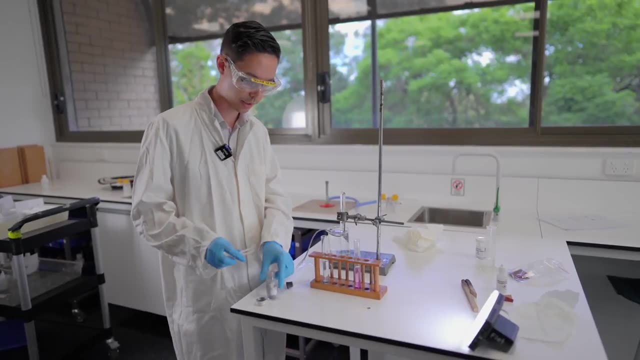 Calcium, now calcium, as you recall from the periodic table that we're showing earlier, it's further down on the the group and we know that the reactivity gets a bit stronger as you get further down the group. so we should see calcium probably will go a bit faster reacting. 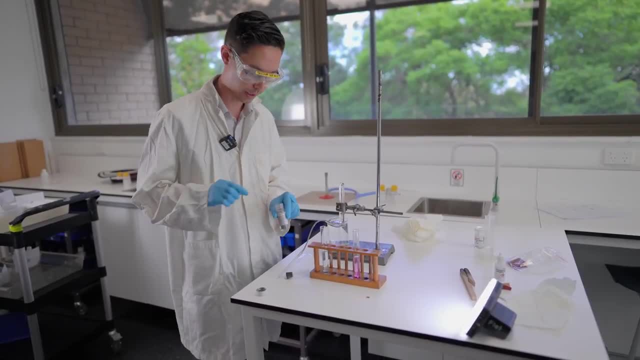 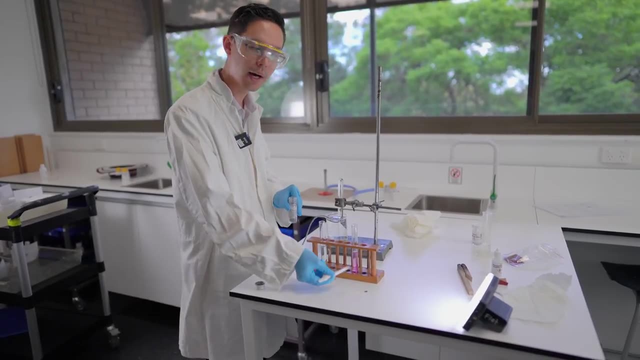 with ordinary water and we won't need to require the assistance of heat to make this happen more quickly. So what I'm going to do this time is that we're going to try and capture the gas that's being produced, the little tiny bubbles we saw with magnesium. so as soon as I drop some in, I'm going to 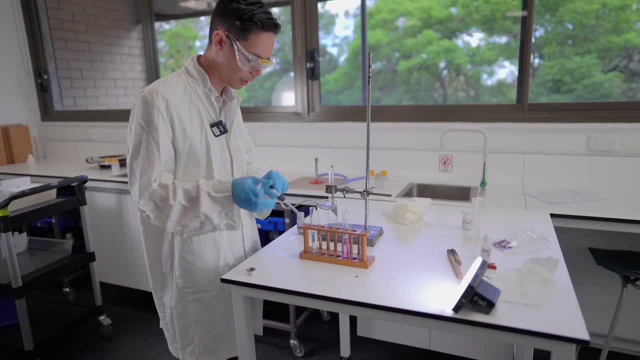 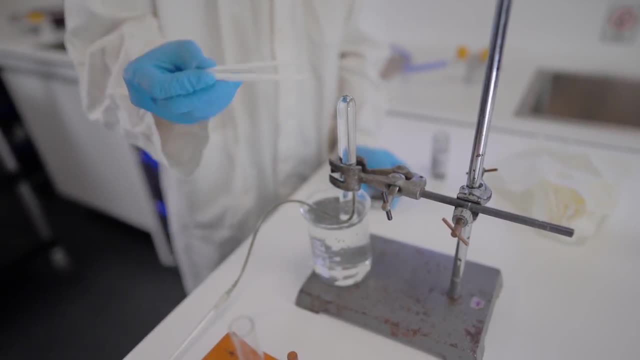 plug it with this. it's a rubber bung with a hole through it and we've got a pipe that leads us to a test tube. we might get my assistant here to get a better view of this test tube here. this whole test tube is filled with water all the 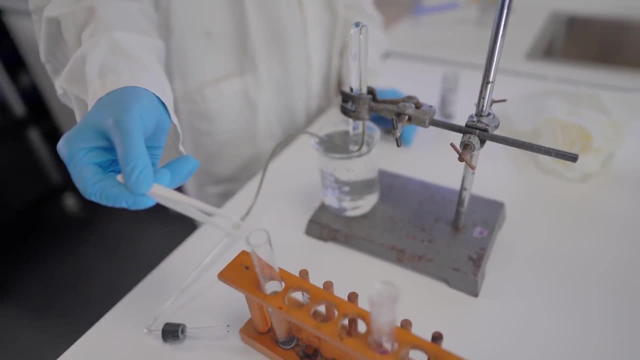 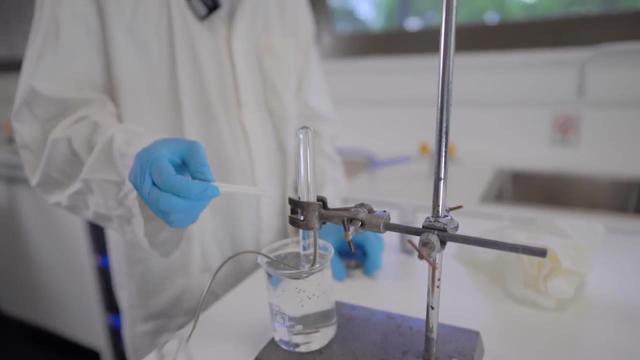 way to the top. so as I produce gas from this test tube, we're going to funnel it all the way up underneath and into this inverted test tube. so any bubbles that are made will start to collect here one by one, and then we're going to do a bit of a flame test to see what kind of gas that is. 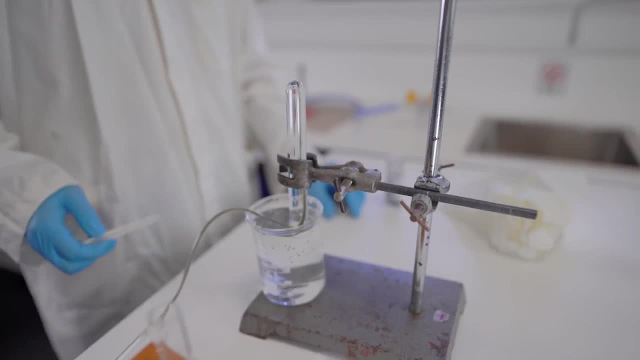 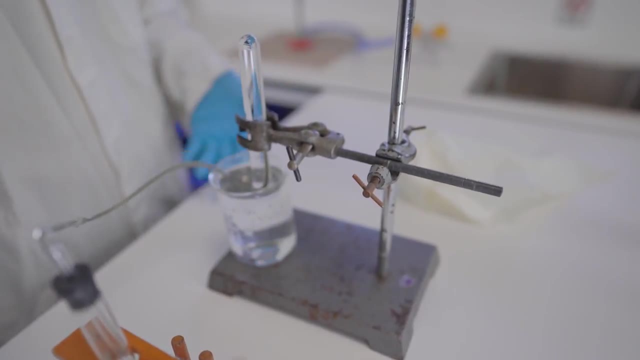 Now I've already given you a bit of a hint that it's hydrogen gas, but Mr Bowman could be wrong. so we could do a bit of a flame test. if it's not hydrogen gas, it could blow the flame out or it could just be a boring result. so we'll find out momentarily. 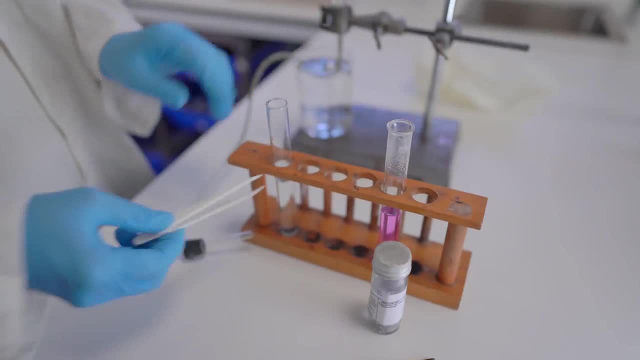 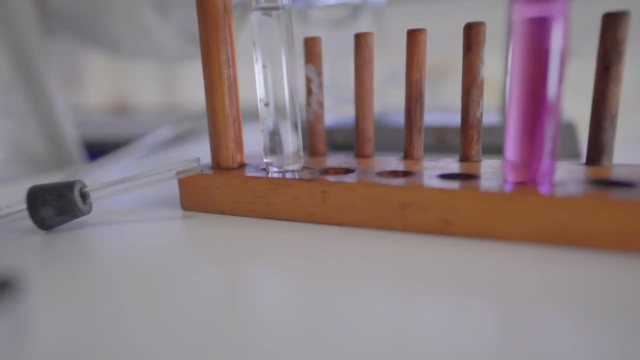 Let's give this a shot. so I'm just going to drop in some calcium metal over here. this is still ordinary distilled water and hopefully the camera can see if there's a change occurring down there. so now I'm going to add the seal and then, if the camera turns its attention to the 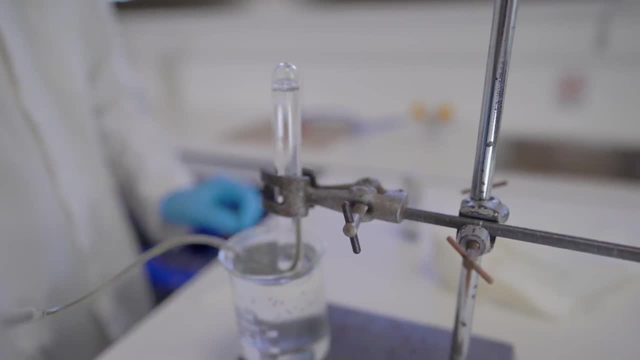 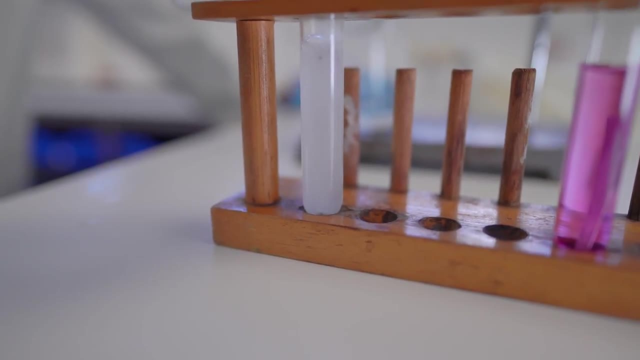 other test tube here. we're just going to keep on collecting it, just keeping some pressure here so the seal stays tight. we're now filling it up with whatever gas is being produced by this other test tube here, which is looking pretty violent. we're nearly filled here, so we 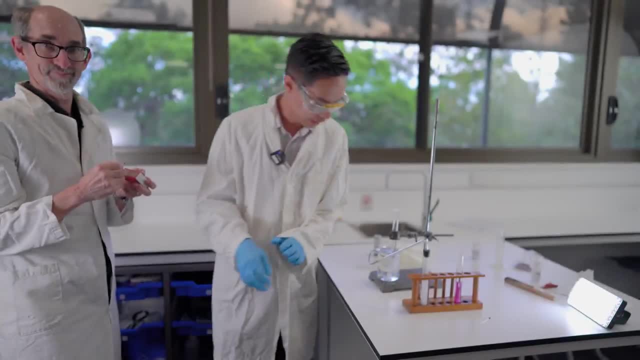 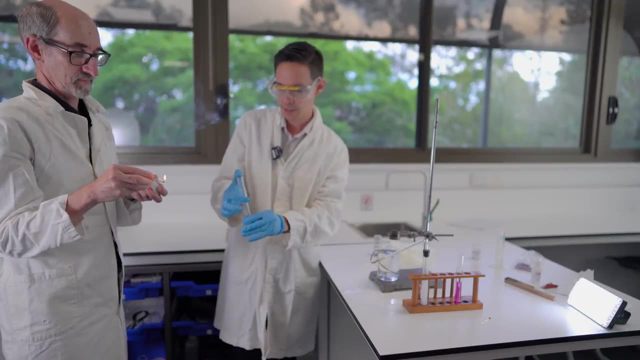 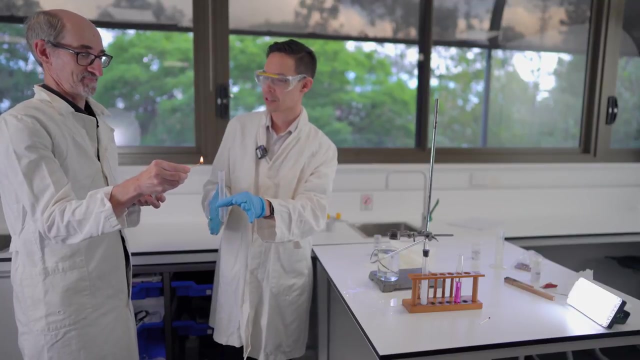 might, um, we might- cut the video. Michael Mayer here giving me some assistance to light my gas on fire, so let me see if I can get the retrieve this. so I haven't let any gas out and on the count of three he's going to put it over the mouth here. one, two, that's definitely hydrogen it. 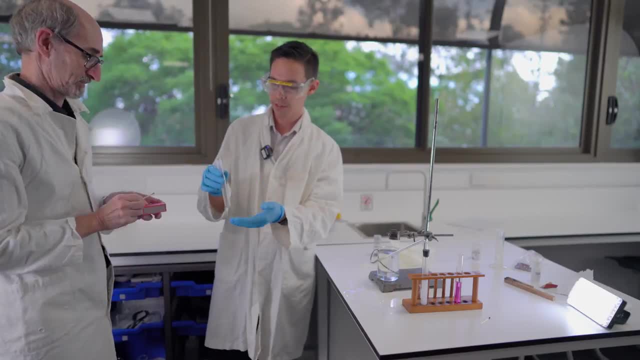 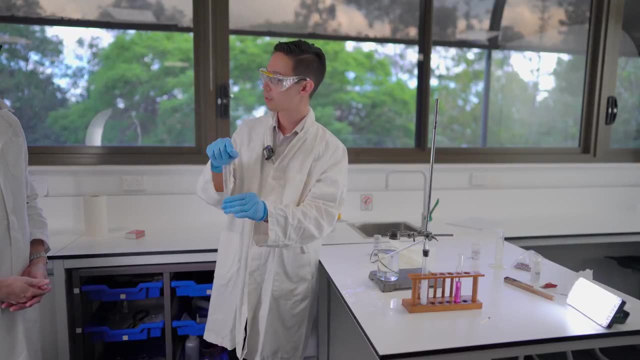 makes this sound it's. you might even get a second. no, you don't even get a second shot. if we had carbon dioxide gas, the flame would just blow out. if the gas was oxygen gas, we should have seen the flame on his matchstick there just flare up and just get more brighter. but this time that sound. 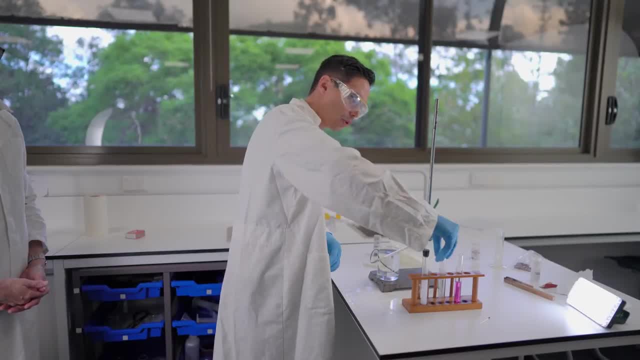 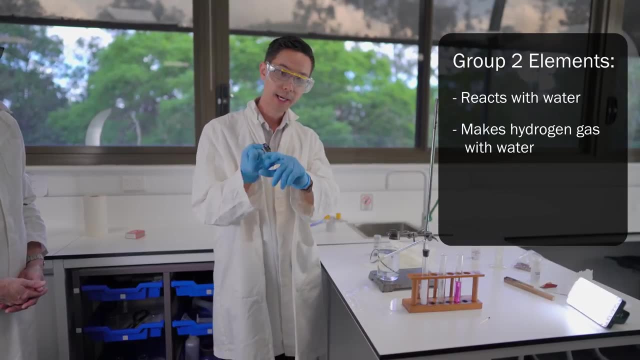 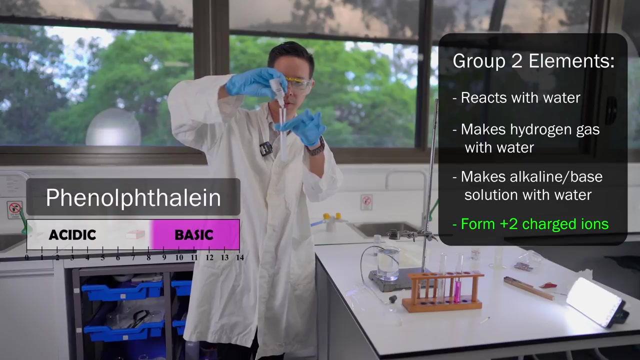 is the characteristic sound of hydrogen gas. so what can we say about the GRIP2 elements? well, they react with water. they react with water to produce hydrogen gas bubbles, and a by-product is that water solution will start to go alkaline. So if I add the phenolphthalein, I should see much more intense pink this time, because we've got far. 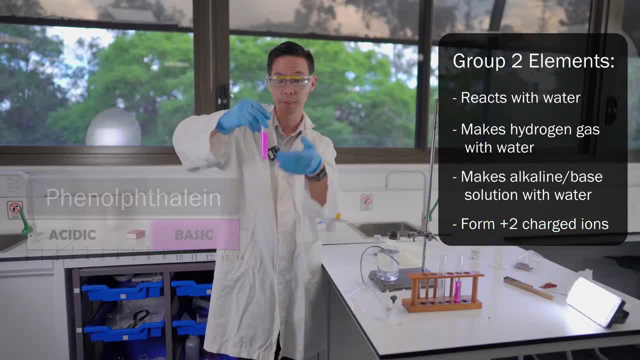 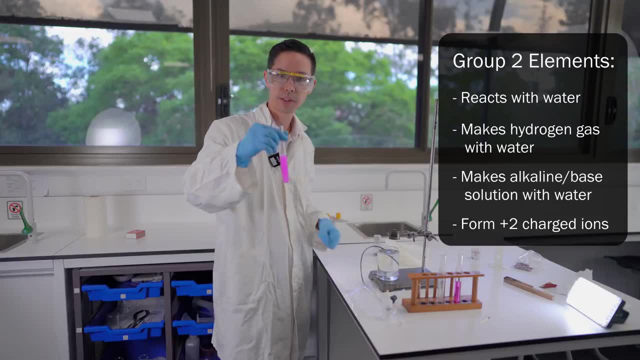 more. yeah, there we go. so we've still got a bit of a a milky appearance because it's creating very many micro bubbles of hydrogen gas. so it's still going. I think that's about it. so that's all I can think of for now. so we'll check in the next video.